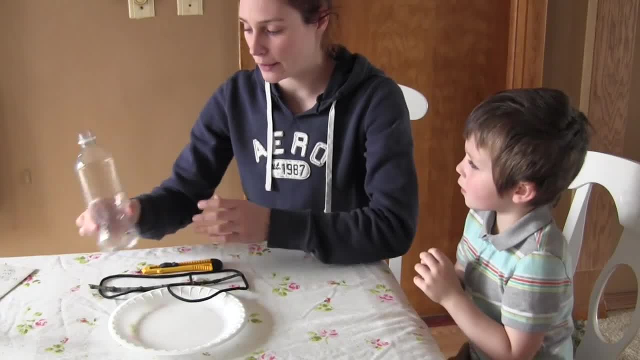 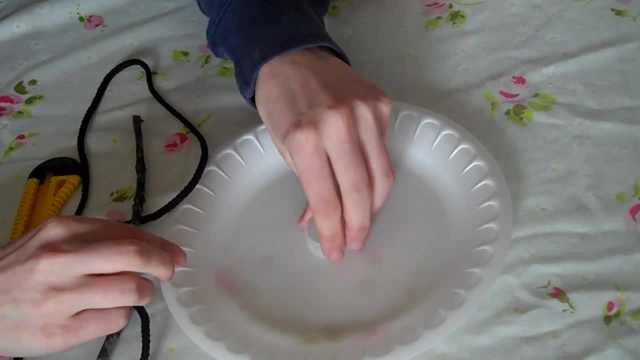 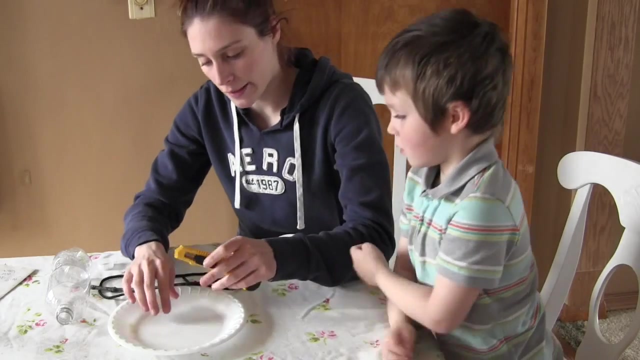 thing we are going to do is we are going to remove the cap from the bottle and, directly in the middle of our plate, we are going to make the outline of the cap and we are going to take our knife and we are just going to cut it out. 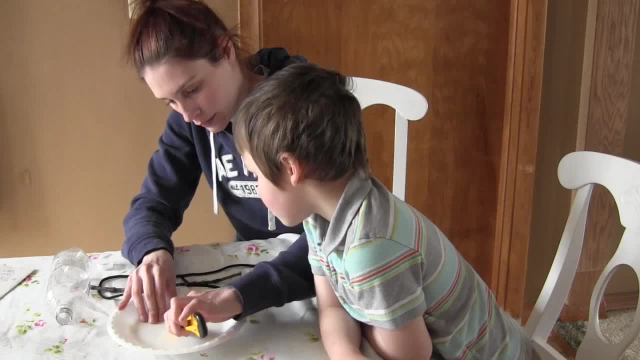 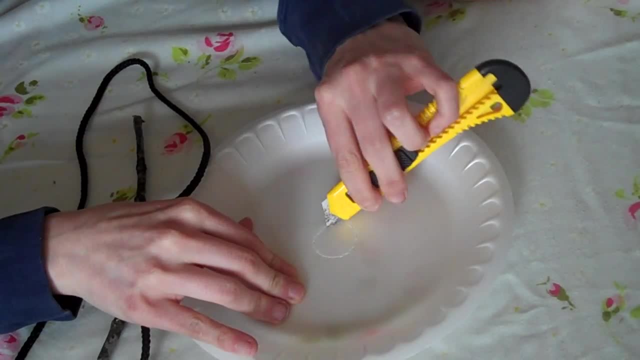 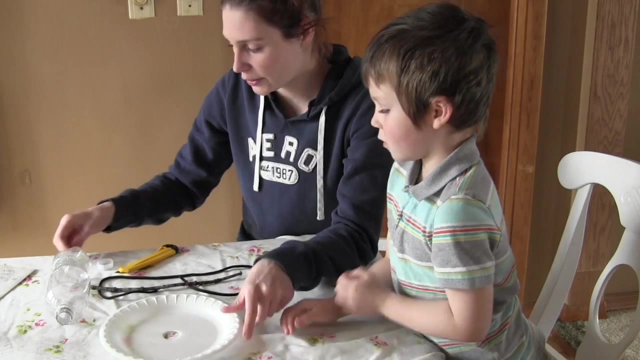 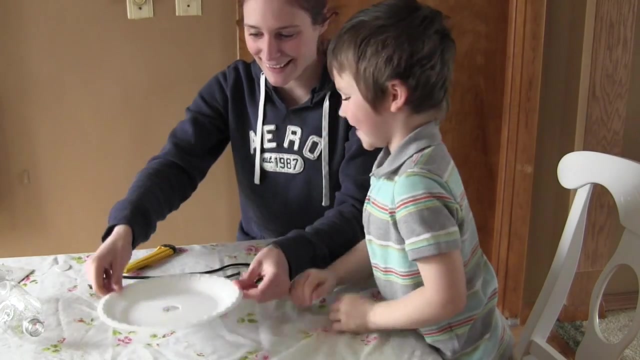 It should be pretty easy to follow the edges. Alright, now this will stand for our birds, to give them a little more stability. See, it has got a hole. There you go. Okay, so the next thing we are going to do is we are going to take our knife and we are going to 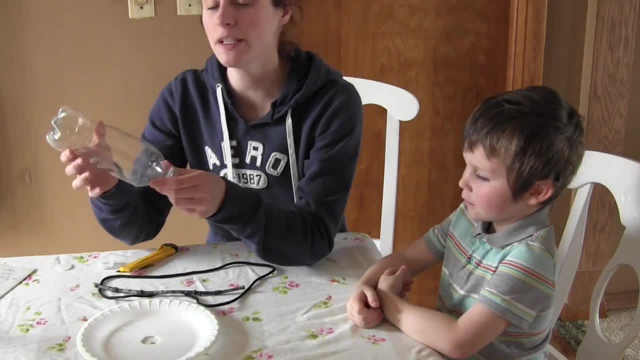 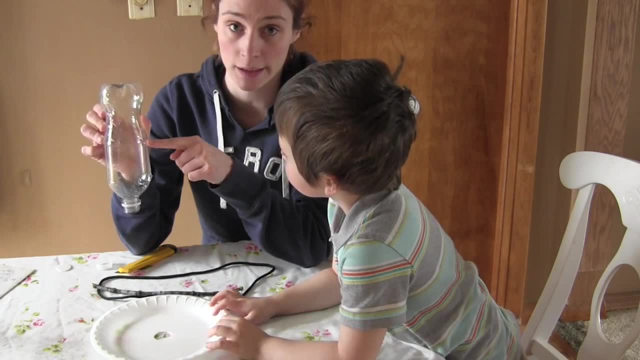 do is we are going to be working with our bottle And in these bottles they have the divider lines where your wrapper used to be around. There is one on the bottom and one on the top. These are going to be our reference points for all of our cuts. So the first cut. 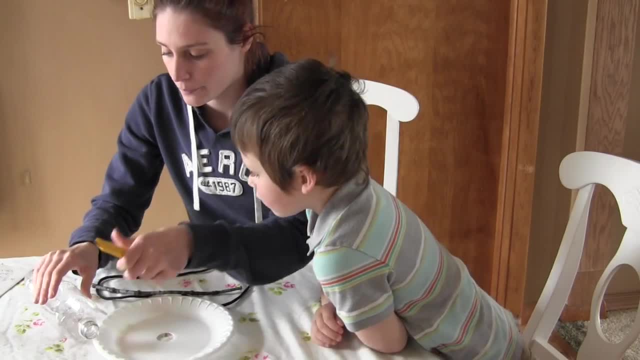 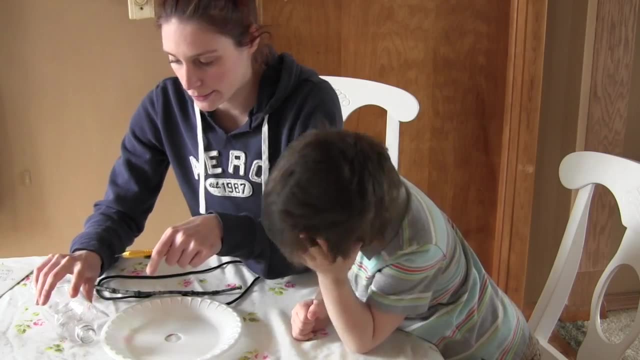 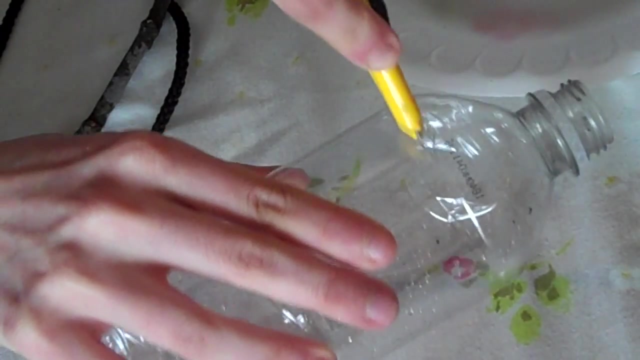 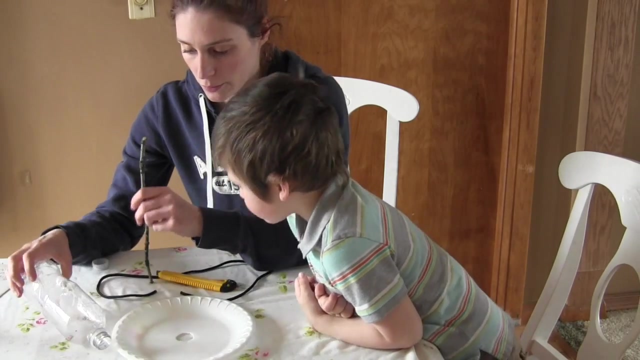 we are going to do is going to be down on this first line. We are just going to stick it through and make a little slit. We are going to do the exact same thing. We are going to put the divider on the opposite side, and this will be for our perch. So we are going. 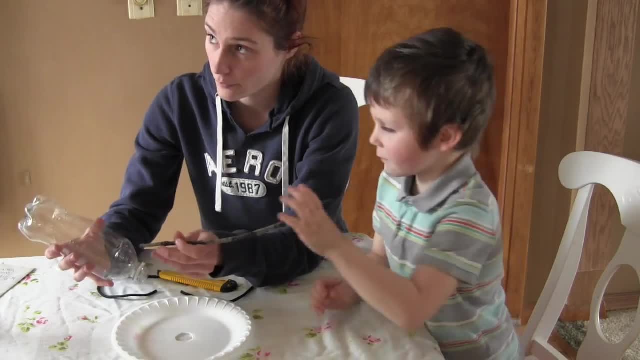 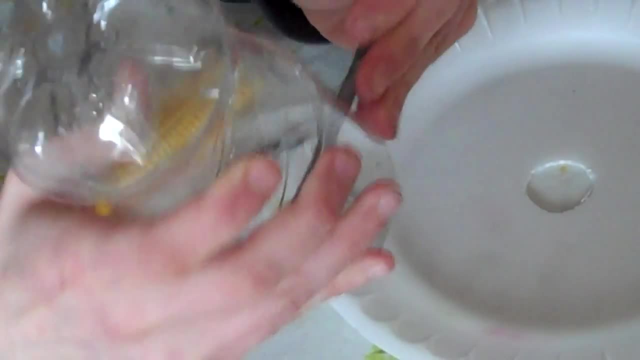 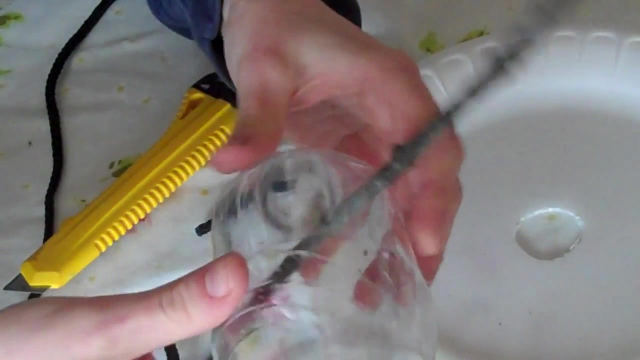 to insert our perch-. do you want to help me get it straight through, all the way across, so that the birds can come to it, So that the birds can perch on it? Okay, and then for our birds to be able to get their bird seed out, we're going to make two little 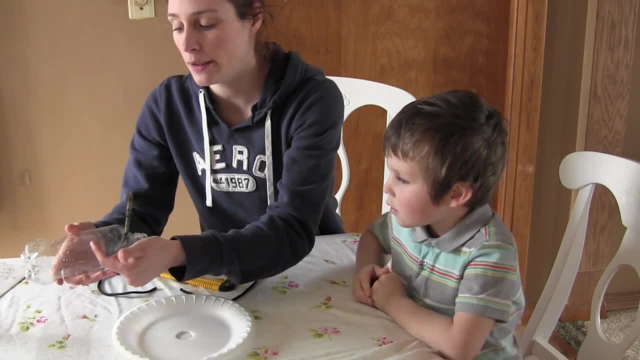 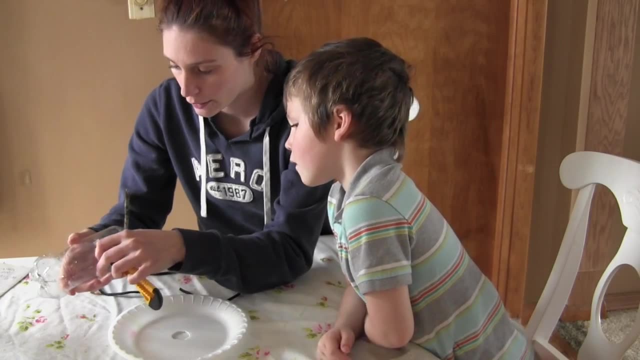 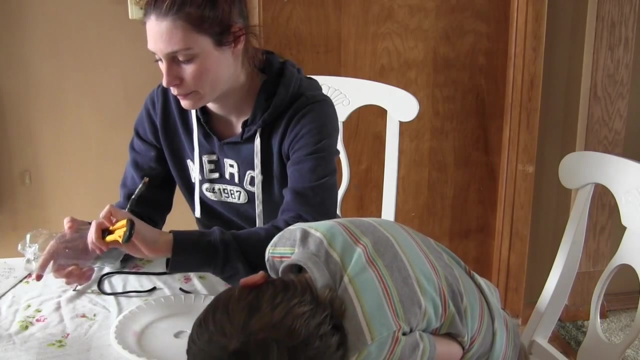 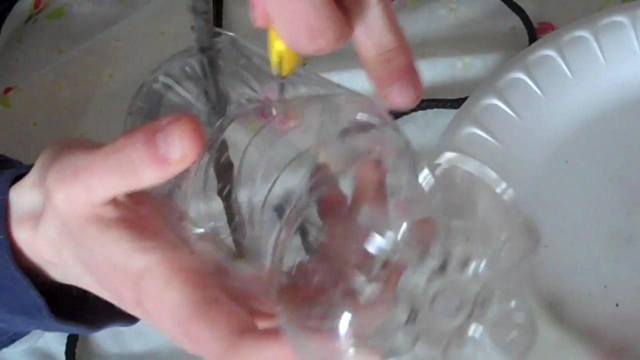 windows for them to pick out of, and those are going to be directly above where the second line, where that wrapper would be. so we're just going to stick it in there. it's going to cut a little triangle and then we'll do it directly on the other side. same thing, it's just a few slits, and if you can't get your, then 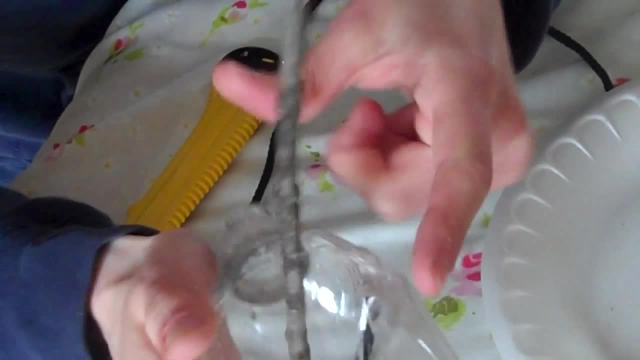 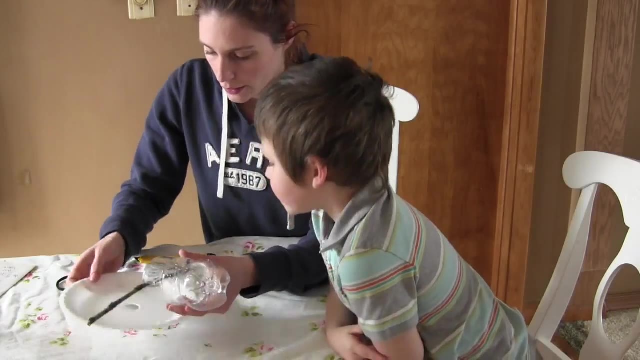 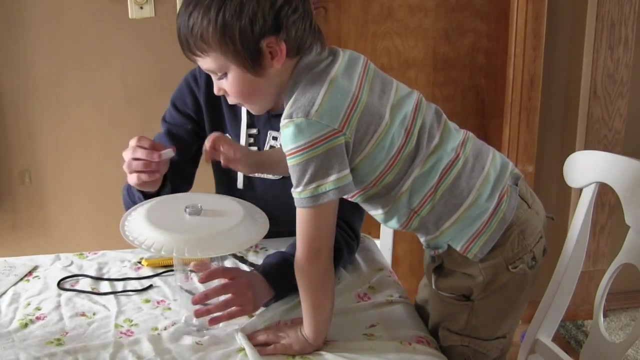 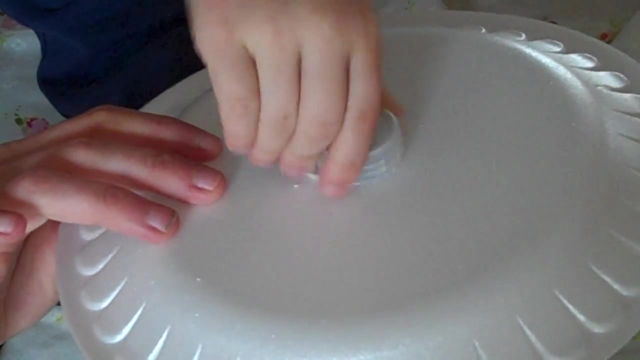 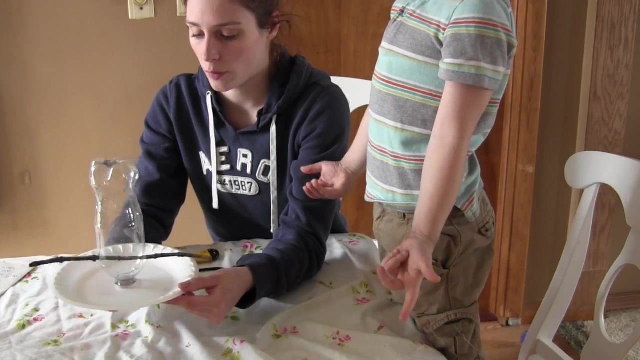 we have our two slits here for a bird to be perched and eating out of their holes, so the next thing we will do then is we will stick our plate through. I'm going to turn it over. Aiden will hi the cap on it. So this is our homemade bird feeder and what we need to do next. 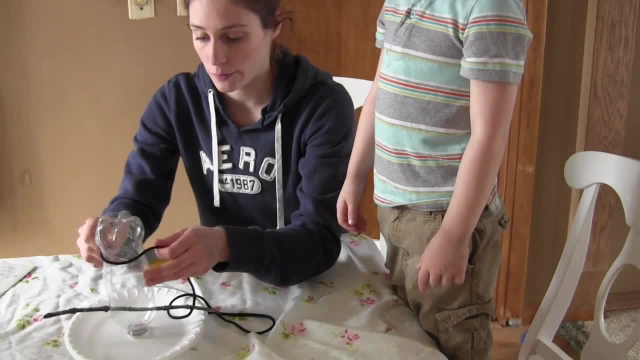 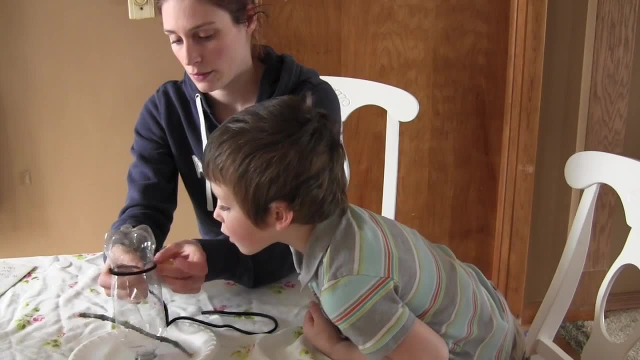 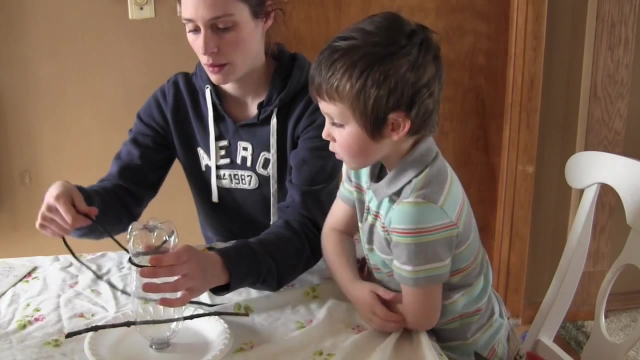 is where our string comes into play is we are just going to take the end of this side, just give it a small knot for now. we'll come back and double knot it. We're going to bring it over the top with a little slack, because this is: 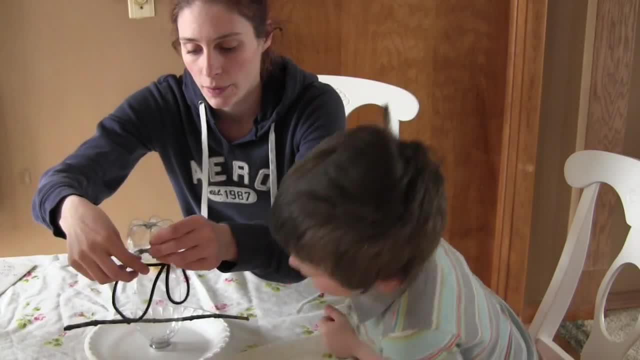 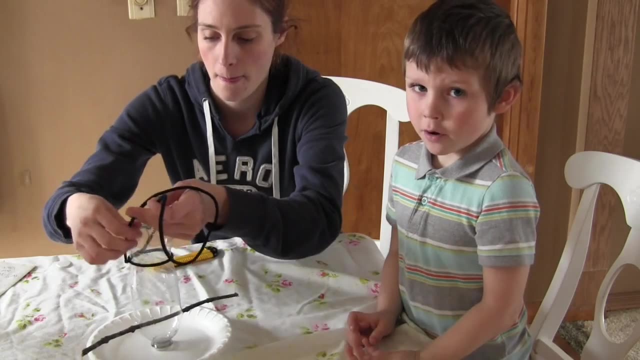 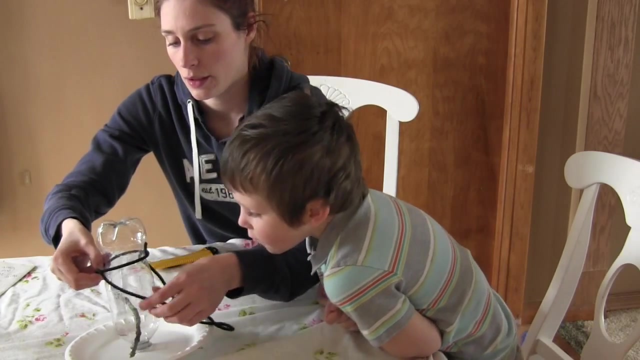 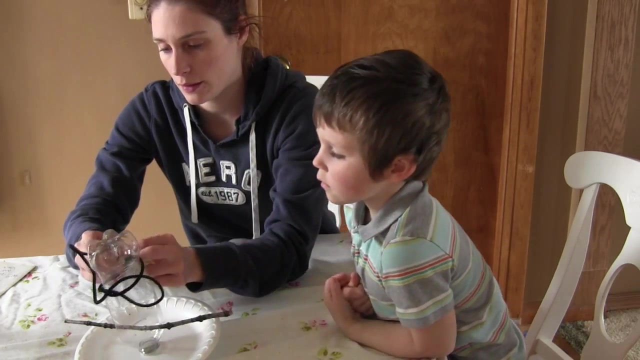 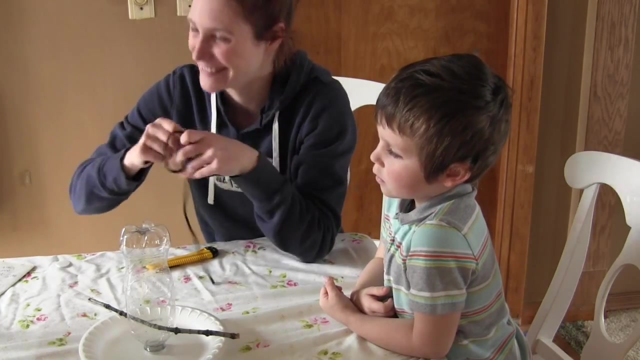 going to be our handle to hang from our tree At our house. we're not going to have a house because we don't want it, So we'll loop the string into the opposite side and make a little knot. She's going to do it again. 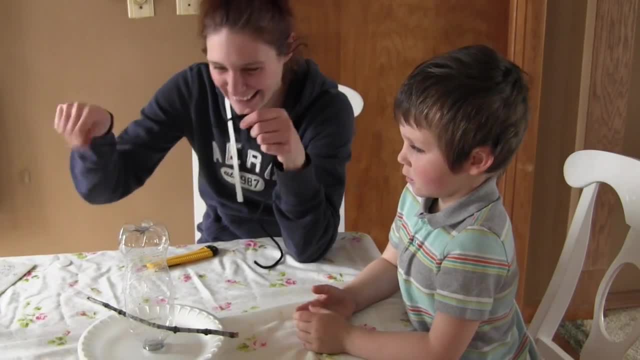 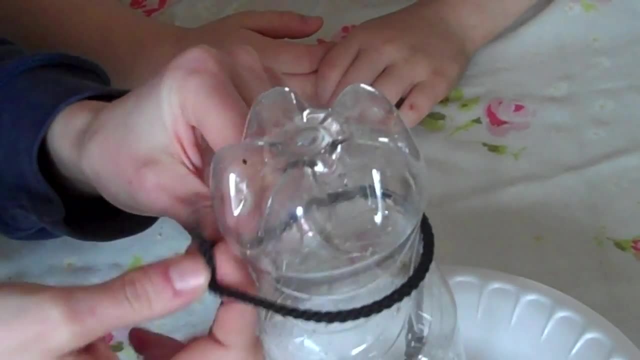 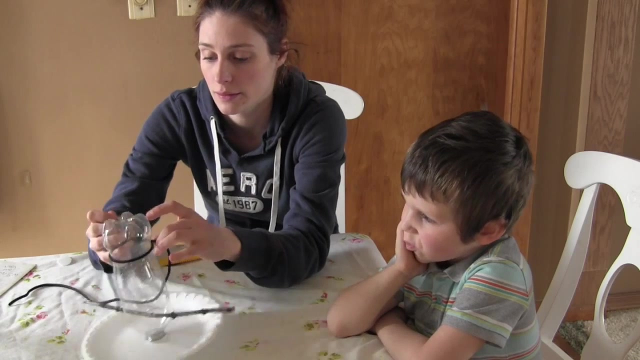 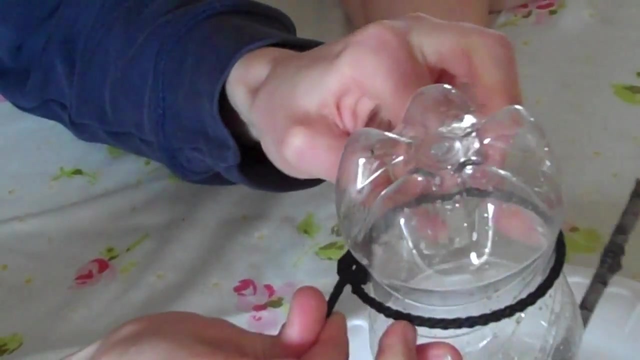 I'm over Cut. We're going to try this again. Okay, It may be a little easier to take the bottle off of the plate to get this to work, but I'm just going to go ahead and double knot this side right away, just so it doesn't fall off. 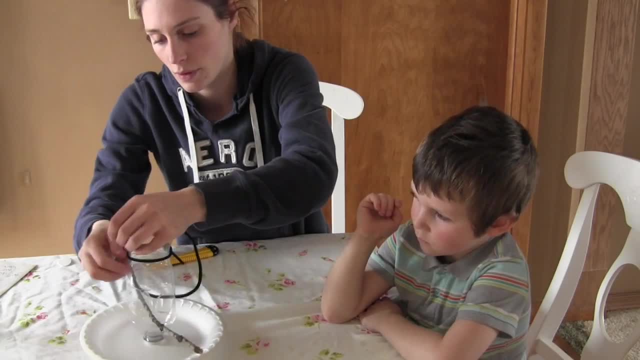 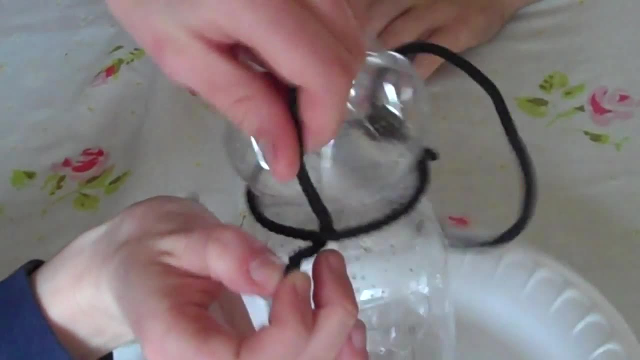 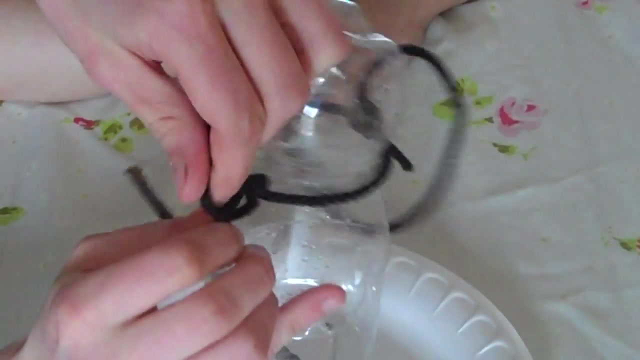 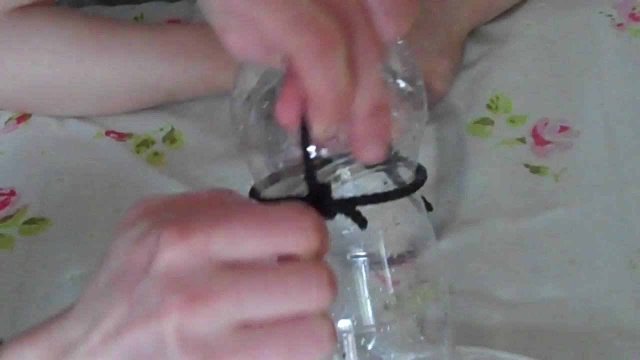 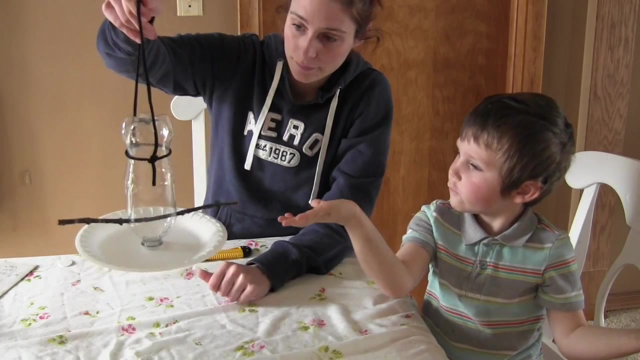 So then we'll take this one and wrap it through our string, Just enough to make a nice double knot. This is a very quick and easy craft to do on even a rainy day when there's really nothing else to do. And this is our finished project. 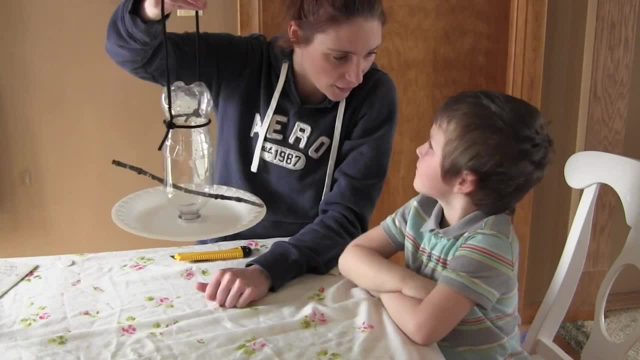 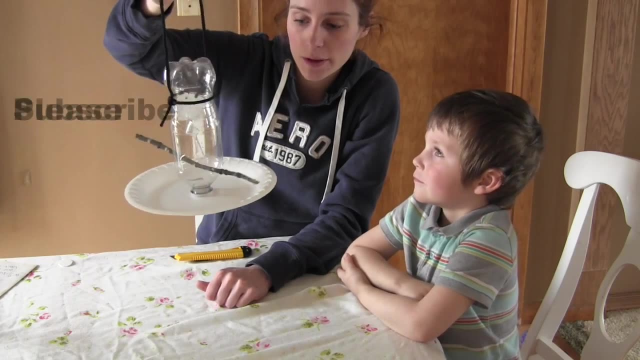 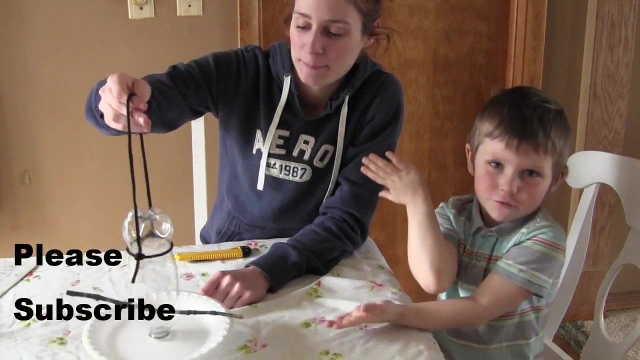 This is our homemade bird feeder from the Pennycrafters Yep and it's awesome. Just hang it from the tree, Put your birdseed in and watch the birds, And when you see them then boom, you look at them.